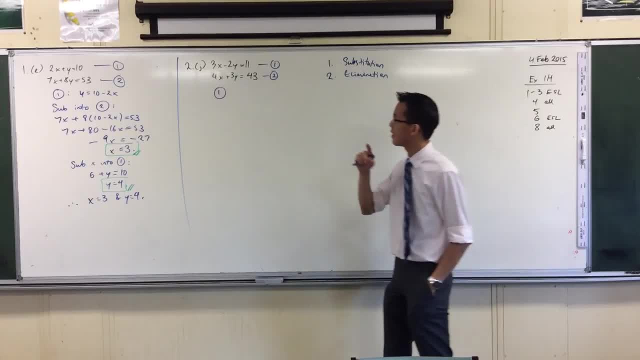 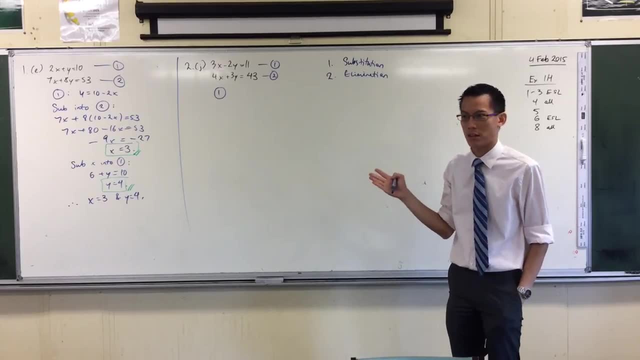 Yeah, Josh, do you want to give it a go? Okay, two and three. let's have a look at this. Why would I multiply by two? How would that be helpful? if I multiply by two, I'm going to end up with 6x minus 4y equals 22.. 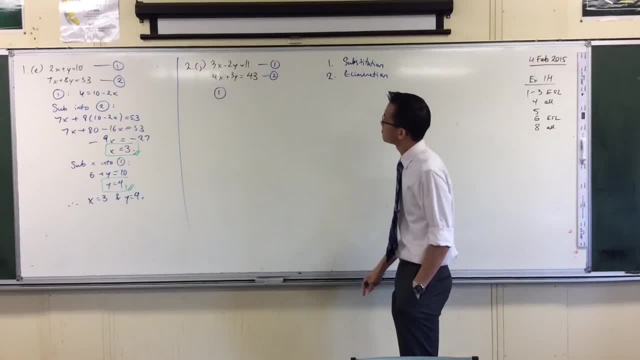 Is that going to be useful to me? Yeah, but it might be useful depending on what coefficients I have in the second equation, right As it so happens at the moment. I look and I see: well, that's a four, that's not going to go to six. 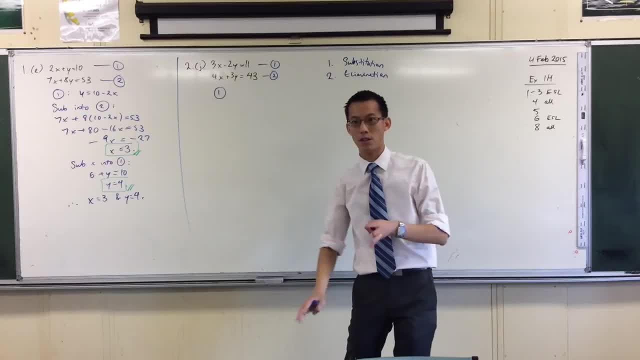 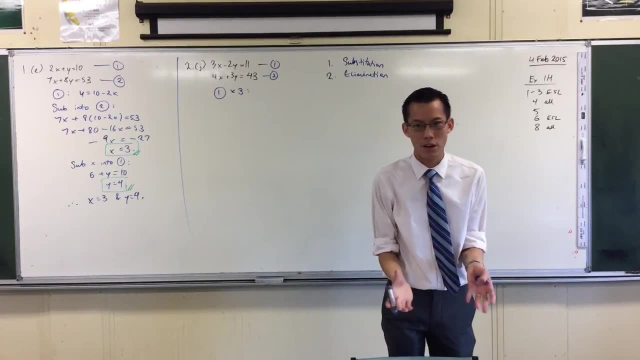 That's a three. that's not going to go to four, so I'm going to need to go to another option Now. the other suggestion was three. Three will work right. Why is three useful? What's the feature about the second equation that's actually going to help me here. 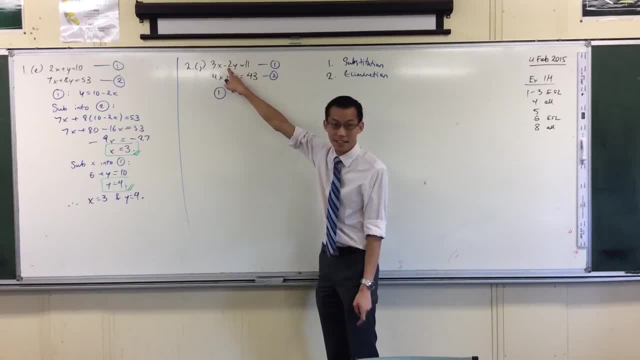 Yeah, right now, Fantastic. So I see that this doesn't have a three in it, but this does. Okay, So three works. What am I going to get? I'm going to have 9x minus 6y equals 33.. 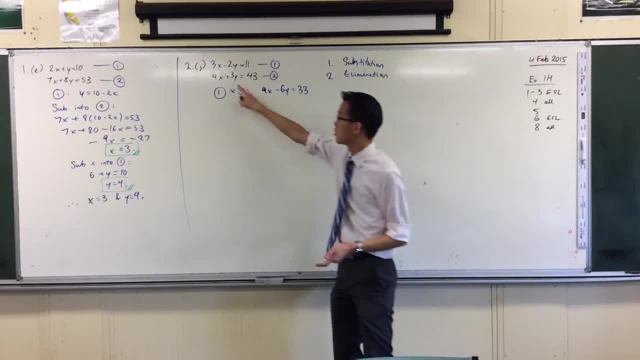 Okay, This is going to work because I'm going to be able to do something here. Now I'm not going to pursue it. You tell me why in a second, why I'm not going to. But what was my other choice? 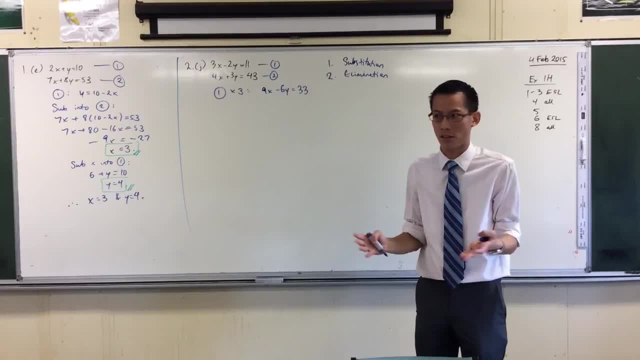 It's not two. What else could I multiply by? that will still work, But it's just not that great. Yeah, four, Very good. I heard it a few times. Four will also work, for the same reason that three will work. 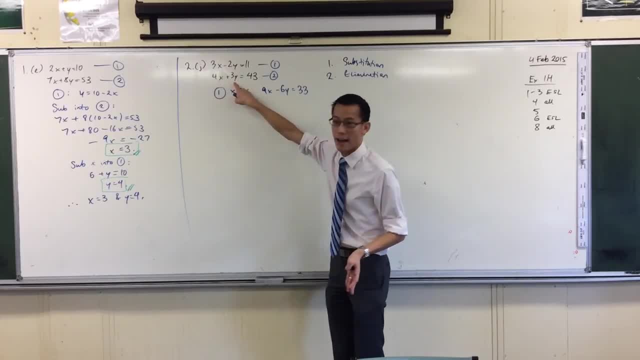 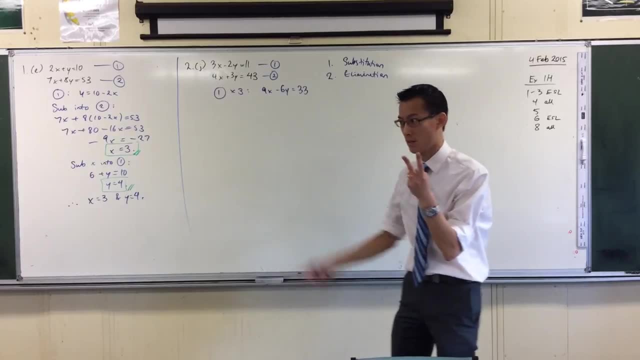 It's just that it will mean I will eliminate. I'm going to avoid that, though I can think of at least two reasons why I'm going to avoid the four. Can anyone tell me why Any one of the reasons? Two reasons: 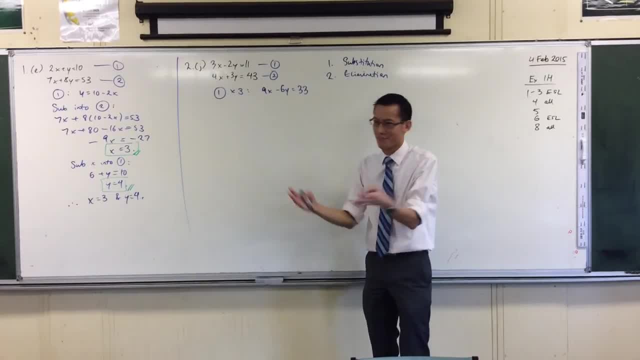 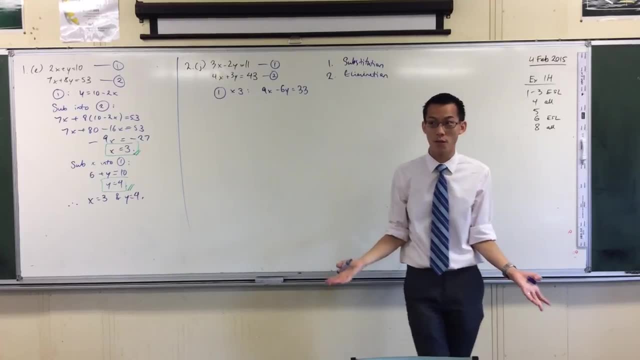 Yeah, Number one it's a bigger number. I know three and four are relatively the same, but they're not always so clean cut Okay. So number one, it's a bigger number. Another suggestion why I want to avoid that: 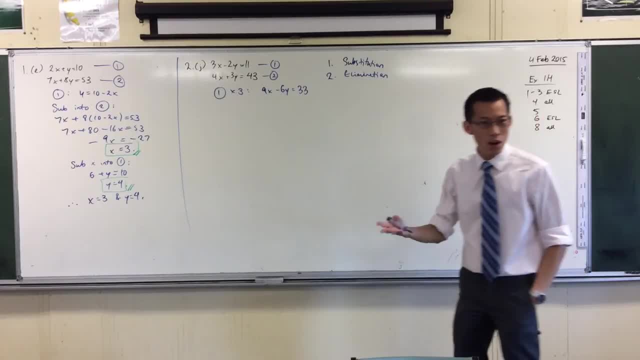 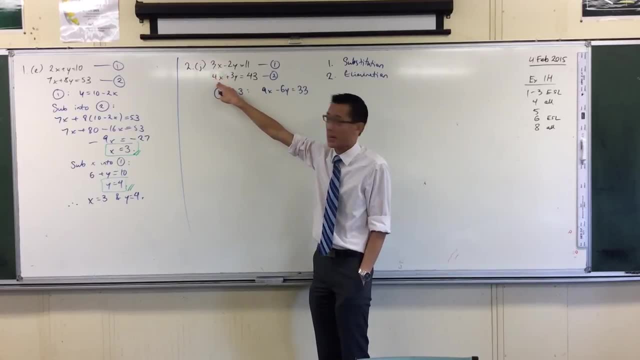 It's a pretty minor one. If I were to multiply by four, then what I'm going to have to do to these two equations is I will have the same number of x's Here and here. I guess I'd have 12x and 12x right. 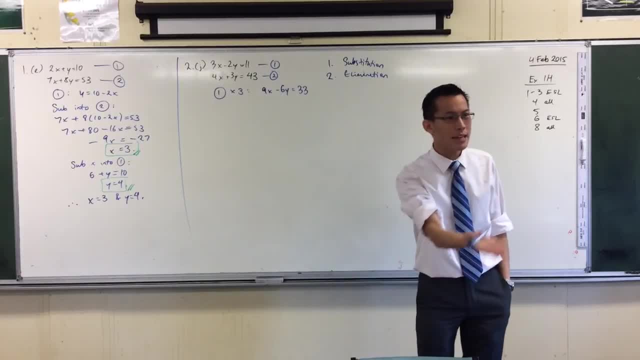 Then I'm going to have to subtract the equations in order to cancel them. Yeah, so I'm going to have to. I'm just going to try. I told you yesterday, right, I avoid subtraction wherever I can, Not because there's anything wrong with it, but because it's error-prone. 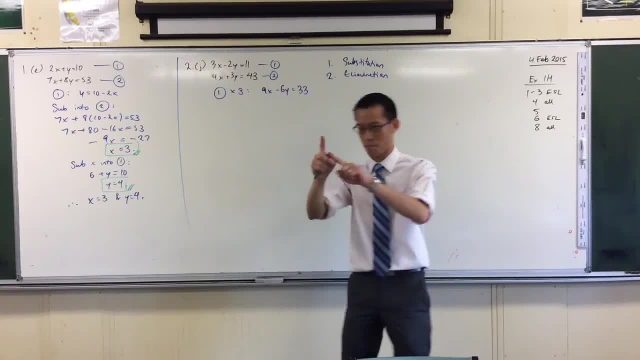 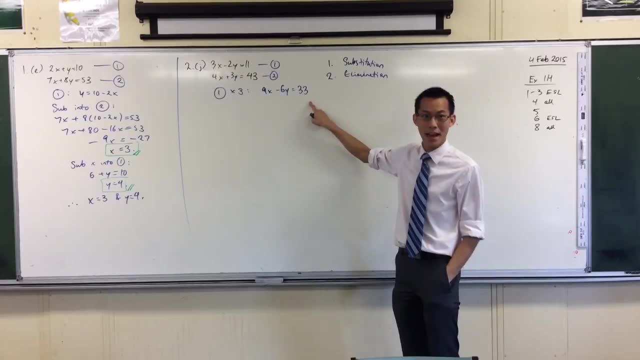 Every time you add in a negative, every time you add in a minus, that's going to multiply by another minus. you're asking to get something wrong. Okay, So that's why this is a better choice. This came from equation one, so can I have a suggestion for what I should name it? 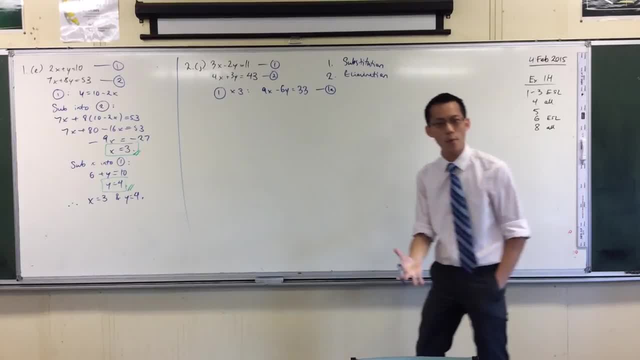 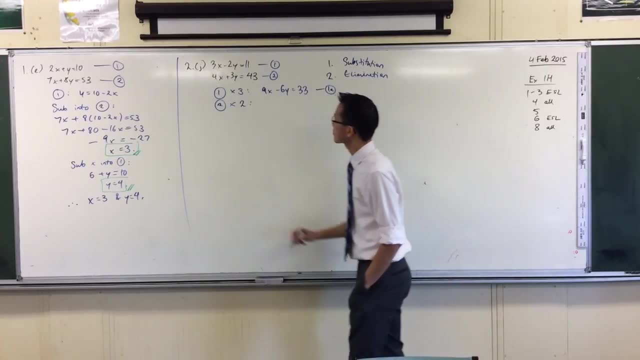 1a- 1a, that's a perfect name, Okay. In just the same way, I'm going to have to multiply equation two In order to have something equivalent. I'll multiply this one by two, Okay. So don't forget to multiply every single term. 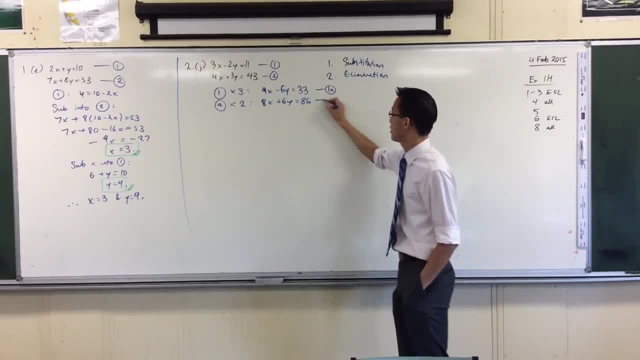 That's another easy error to make when you're doing the elimination method. Being that that came from equation two, I'll call that 2a. So now my stars have aligned. I have the negative, the minus 6y here, the plus 6y there, so now I'm just going to 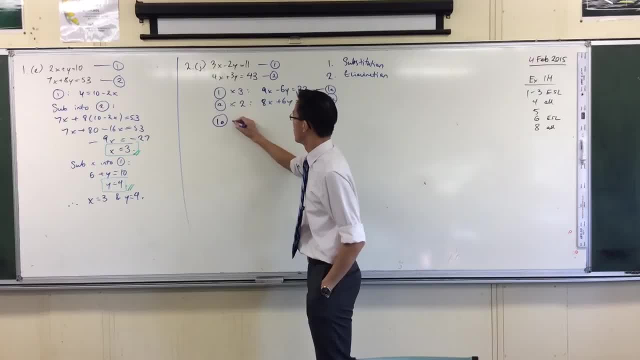 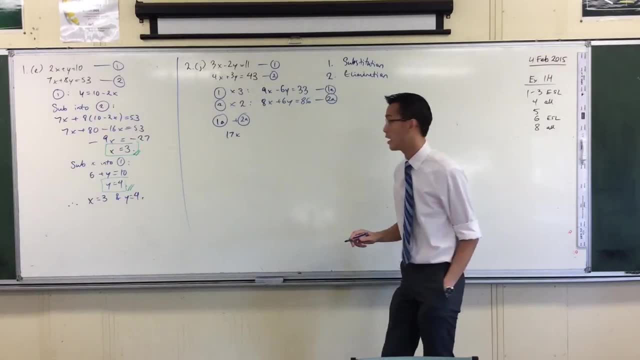 Add the equations to the other. Adding is always a better way to go, So I'm going to get- excuse me, 17x here. My y's cancel. What do I get on the right-hand side? 119.. Okay. 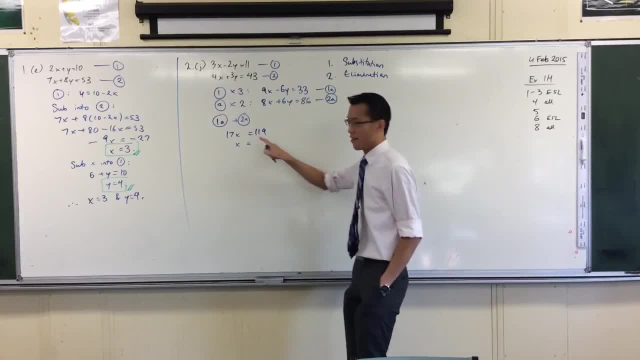 So x is going to be equal to Now. before you look at it and think, oh, I need my calculator for this one. Okay, Sure, get your calculator eventually, But you need to exercise that muscle, Otherwise it's going to atrophy. 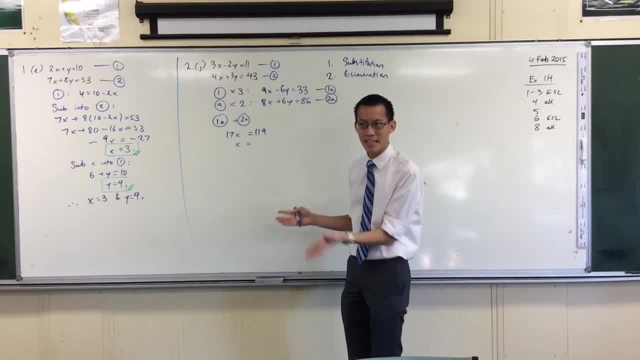 And there's an easy way to see it must be 7, right? What's the easy way to see that it must be 7?? It's the 9. Because you look at the 9. You're like what can multiply by 7 to give me a 9 on the end. 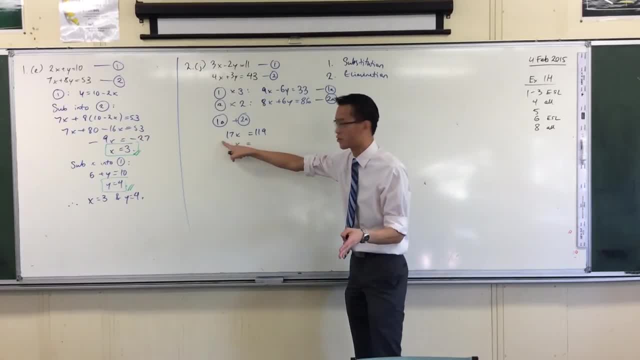 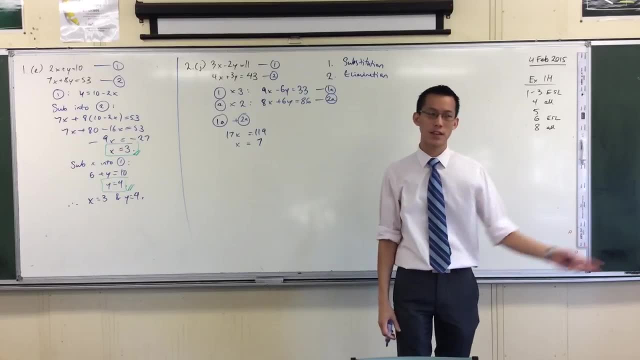 It would be: 7 times 7 is 49, right? And then I've got some extra. And then you mentally check it out: 70 plus 49. Yeah, it works. Okay. So it's an easy division. Don't reach for the calculator if you don't have to. 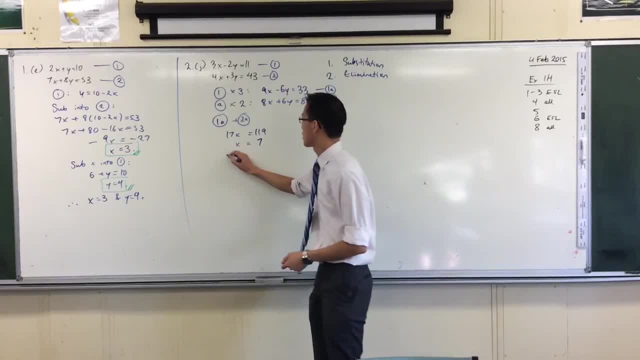 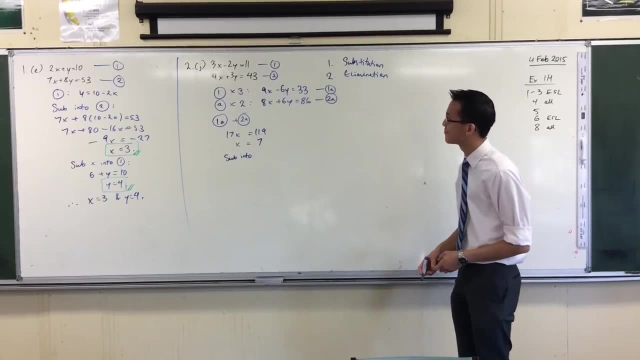 Okay, Just like before, I'm going to take that and I'm going to substitute into Any suggestions. What do you think is the best way? I actually think it's kind of equal here. One gives you smaller numbers, but you've got a negative. 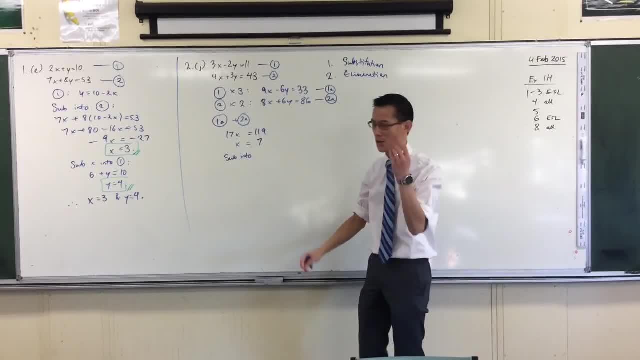 Two gives you bigger numbers, but everything's positive and nice and neat. Just because you asked for it, let's put it into 1.. So what am I going to get there? 21. Yeah, So I've got a negative 10 over there.